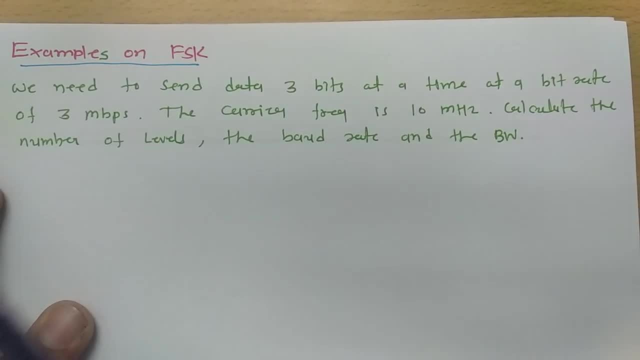 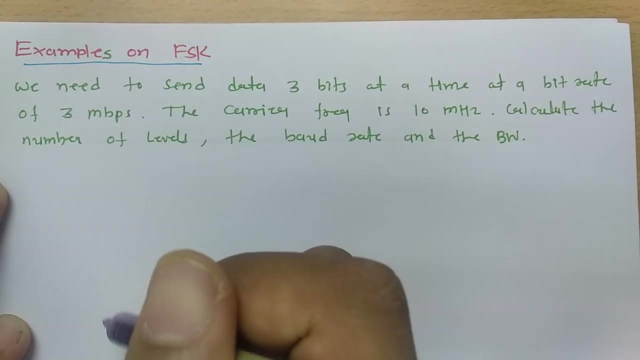 Welcome to digital communication playlist. Here in this session, I'll be solving examples on FSK and I'll request you, before you solve these examples here, you should see my previous video based on FSK, where I have explained all the basics regarding FSK and that will be so essential to 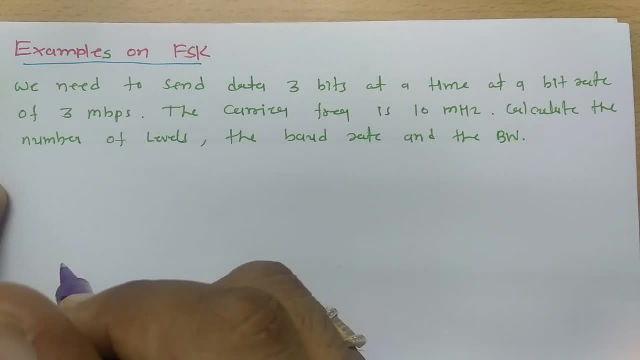 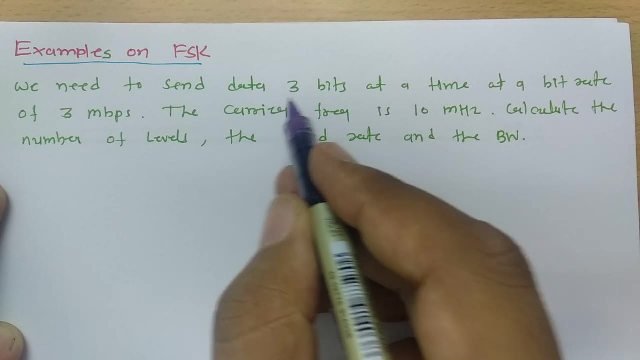 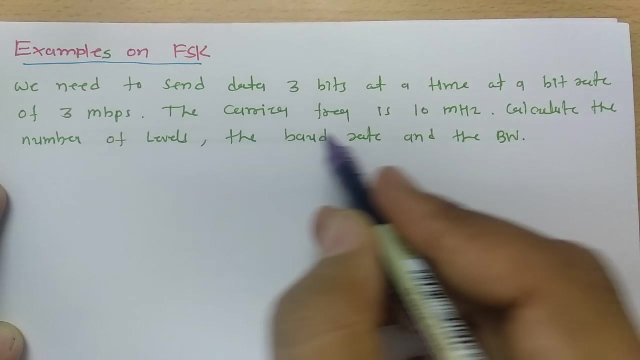 solve these problems, which I am doing it over here in this session. So let us begin this session with first problem, where, see, we need to send a data of 3 bits at a time at a bit rate of 3 Mbps. The carrier frequency is 10 MHz. Calculate the number of levels. 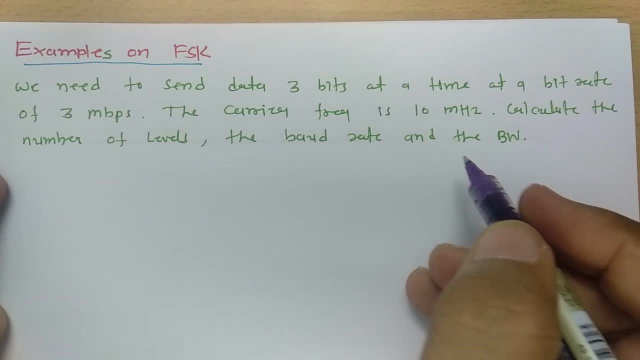 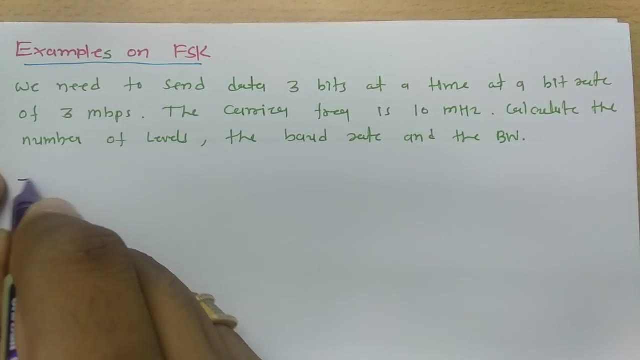 baud rate and the bandwidth. So here we are dealing with to calculate three things: levels, baud rate and bandwidth. So see, first of all, let us mention all those data and then we will be able to solve these problems. So let us begin with the first problem where see. 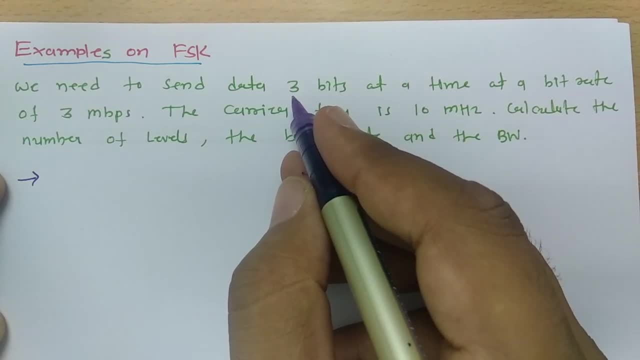 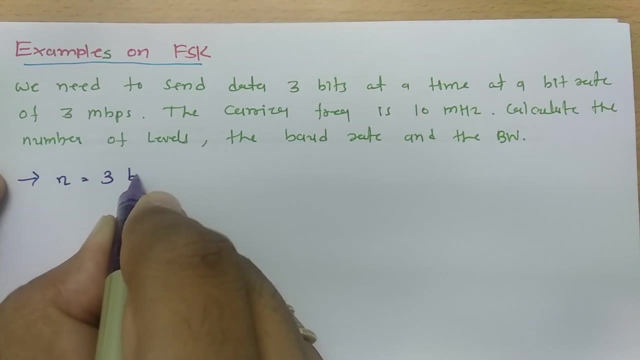 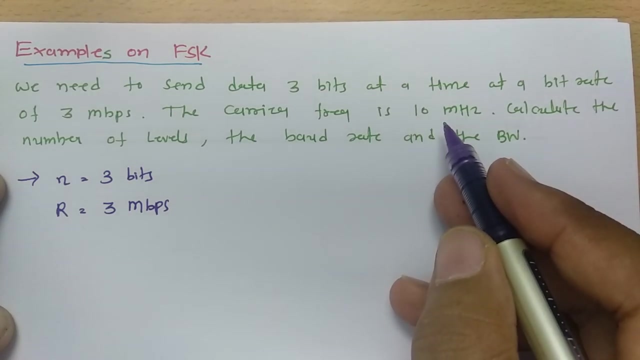 which is given to us. So here, three bits, that is what we are delivered to send at a time. It means small, n is given, that is three bits, with the bit rate of 3 Mbps. So data rate is given capital R, that is 3 Mbps, and the carrier frequency is of 10 MHz. So carrier frequency at C, that is given. 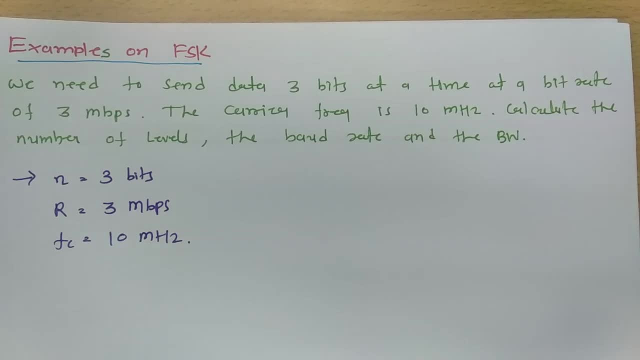 10 MHz. So we are delivered to identify first number of levels. So let us calculate number of levels. L is equal two to the power, n, and here n is equal to 3. So it is 8. so total 8 number of levels are there. 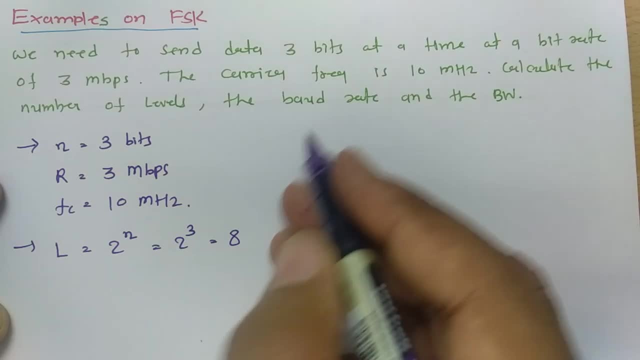 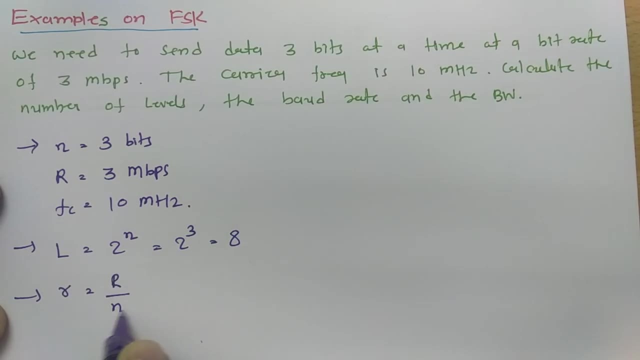 Now we are delivered to identify opioid rate. Now see the relation in between baud rate and bit rate is: baud rate is equals to bit rate divided by n. now see bit rate. that is given 3 mbps and n is given 3 bits. so 3 mbps divided by 3, that is 1 m baud. so baud rate is. 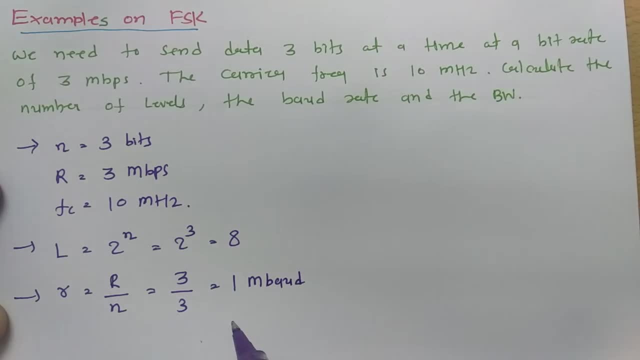 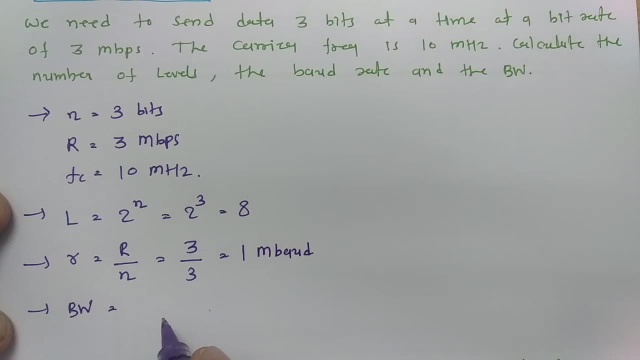 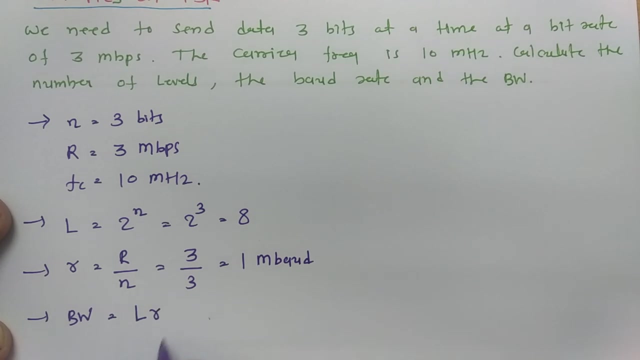 1 mbps. now, third is we are delivered to calculate bandwidth. so see minimum bandwidth that i have already explained. for l level, fsk, minimum bandwidth will be l into r, where l is number of levels. there are total 8 levels. so here we have 8 levels. into r is baud rate. that is 1 mbps. 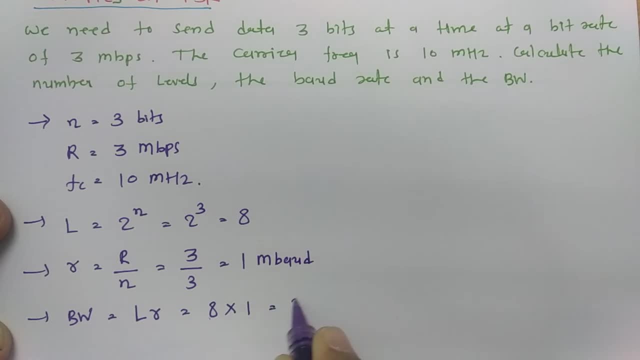 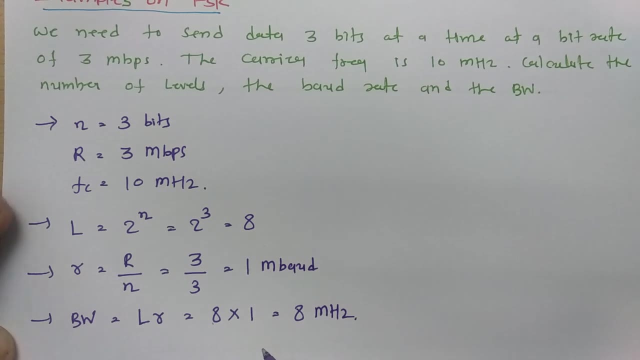 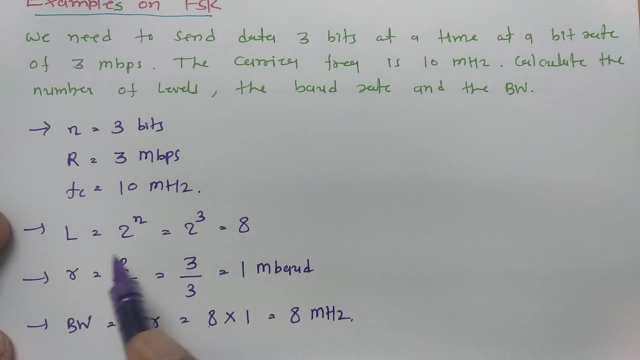 so 1, 1 mega. it means it is 8 megahertz, so bandwidth will be 8 megahertz. so see, these are the basic things that we need to understand based on previous theory sessions, which i have done. so number of levels is 2 to the power n relation between baud rate and bit rate is. baud rate is 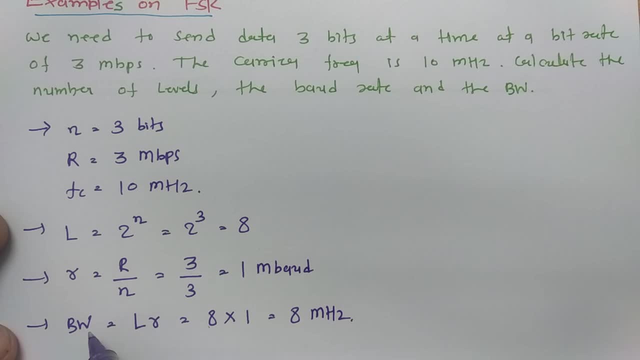 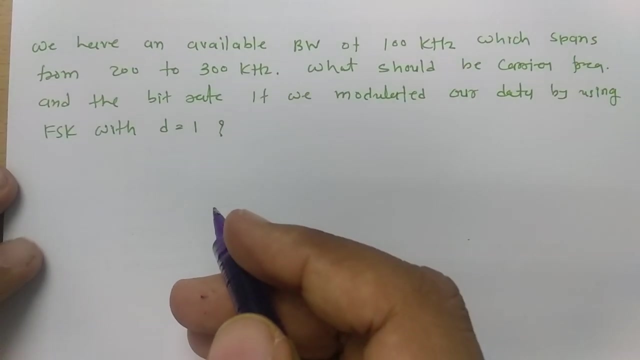 equals to bit rate divided by n and bandwidth for l level, fsk, that is l into r, where l is number of levels and r is baud rate. so this is of. we can solve this problem. now let us have one more problem. see this: we have available bandwidth of hundred kilohertz. 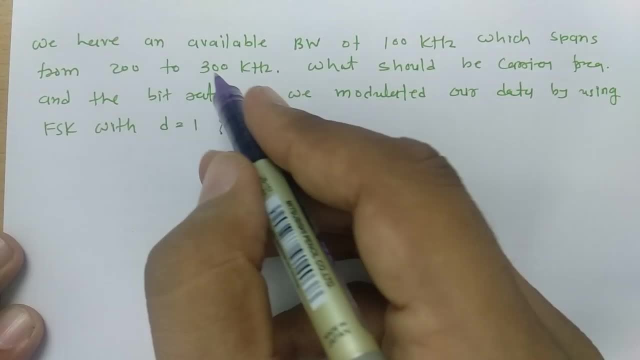 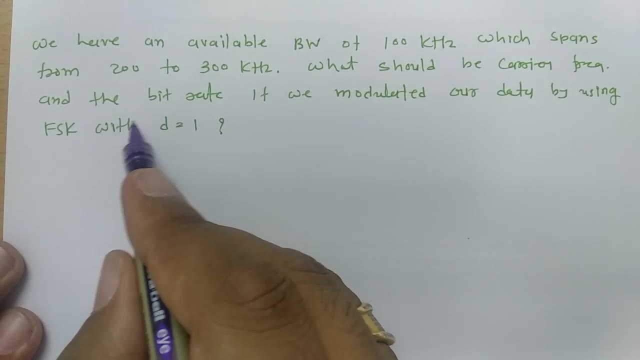 which spans from 200 to 300 kilohertz, what should be carrier frequency and the bit rate. if we multiply this by number of levels as well as bandwidth, we get this meshed. band-ithe diameter are called batt pimple. here it is 0.5Khz, which spans from 1 kHz, which is 0. modesל and else. So if we need each band volume, we get the sum of. 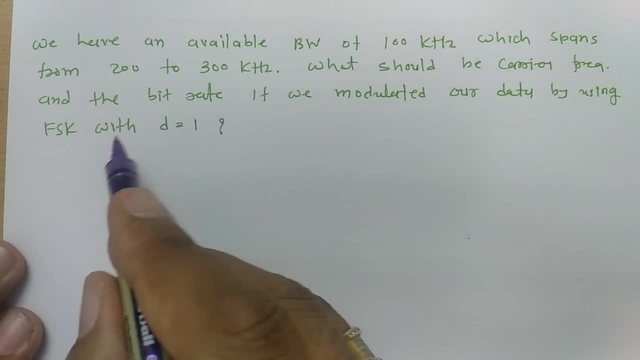 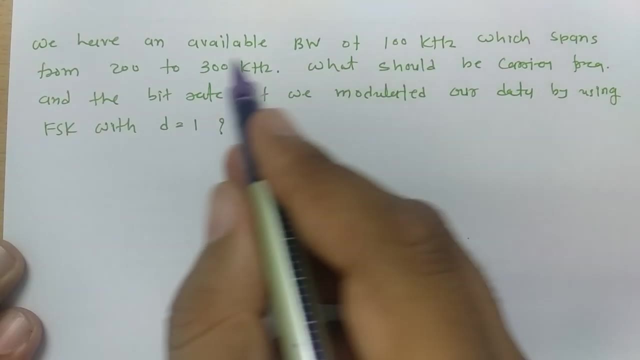 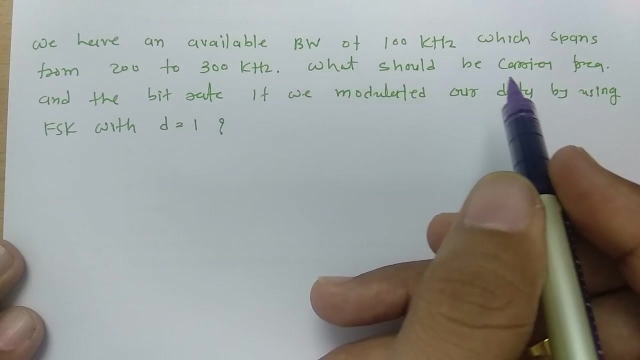 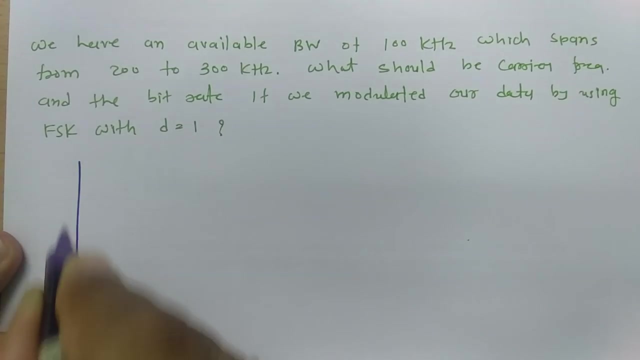 we modulate our data by using fsk with d is equals to 1, so we have bandwidth of 100 kilohertz and that is spanned from 200 to 300 kilohertz. question is, what should be the carrier frequency? and that is there in fsk, so let us plot that first in fsk. so here we have frequency. 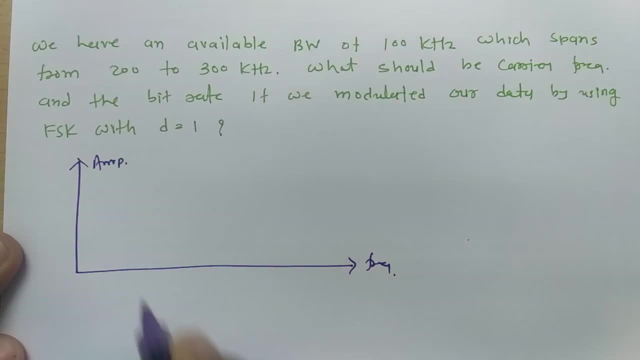 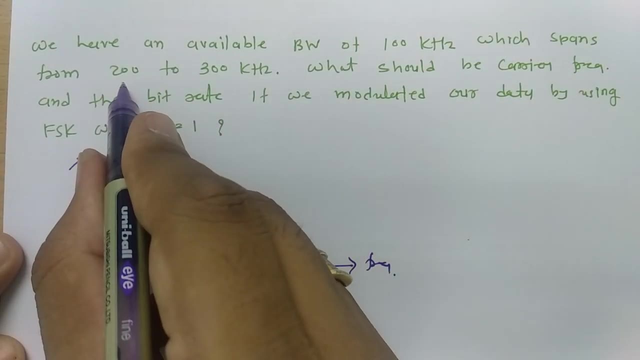 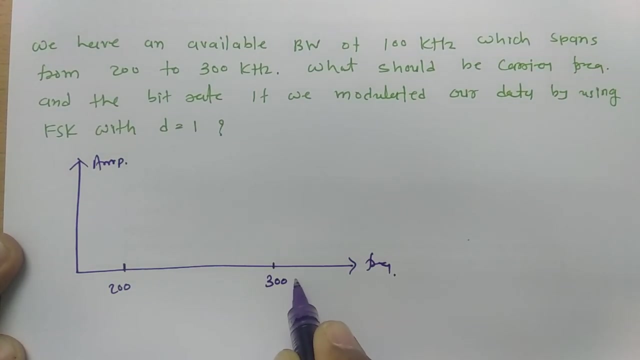 here we have amplitude. now see in f. in this fsk bandwidth is given from 200 to 300 kilohertz. so if i say here there is 200 and here there is 300 kilohertz, so basically what will happen is like there are two frequency carriers that we are delivered to. 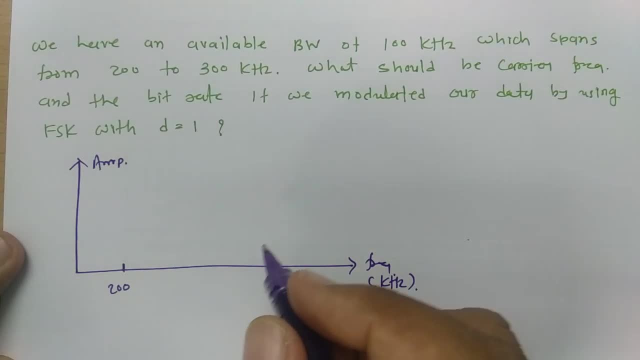 send in. so basically what will happen is like there are two frequency carriers that we are delivered to fsk. one is for zeros and one is for ones. so when you bisect this, so center will be over here, so center will be 250 kilohertz, so one band that will be observing. it is happening like this: 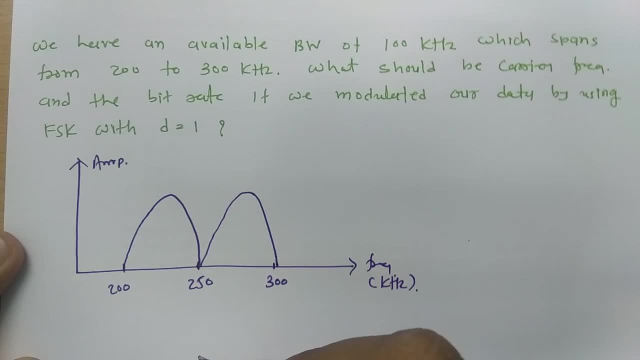 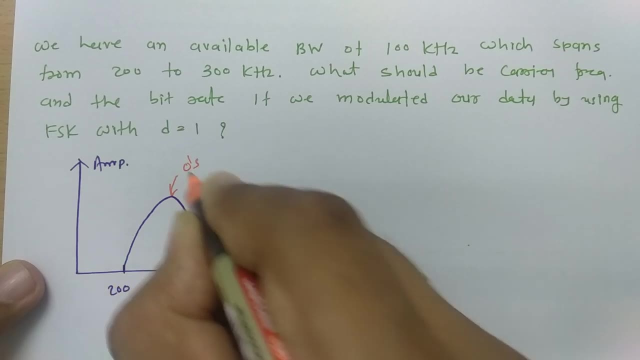 and second band. that will be happening like this: now if i say this band that is there with zero. now if i say this band that is there with zero. now if i say this band that is there with zero zeros in this band that is there with ones. 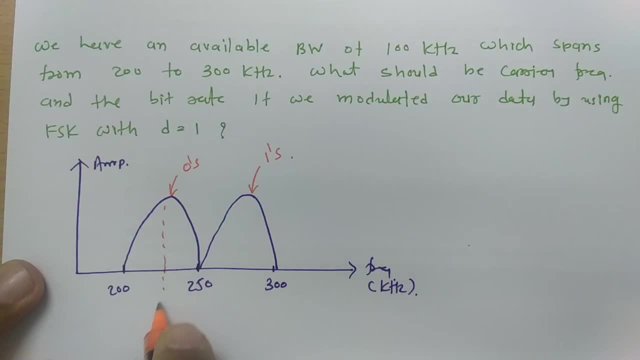 zeros in this band that is there with ones. zeros in this band that is there with ones, then its center frequency that will be over here, then its center frequency that will be over here, then its center frequency that will be over here. if i say this is fc0, then fc0 has to be. 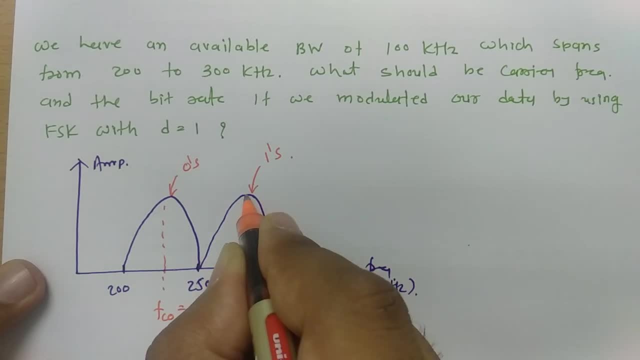 if i say this is fc0, then fc0 has to be. if i say this is fc0, then fc0 has to be: 225 kilohertz, 225 kilohertz, 225 kilohertz. and if i say this is second wind, that is. 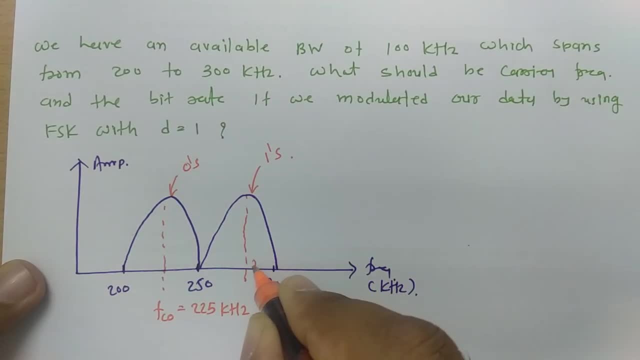 and if i say this is second wind, that is, and if i say this is second wind, that is there with ones, there with ones, there with ones, so its frequency will be, so its frequency will be, so its frequency will be fc1 and that has to be in between this. 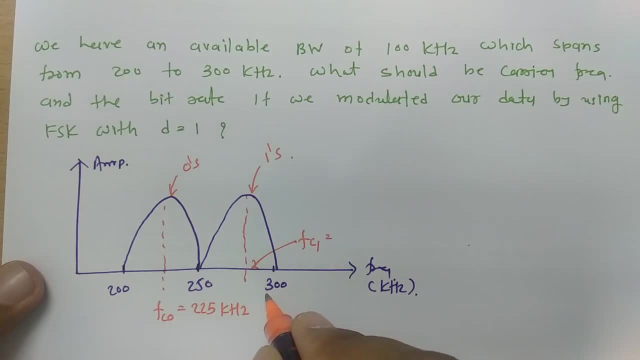 fc1 and that has to be in between this fc1 and that has to be in between this two 250, two 250, two 250, and in between 250 and 300, so that has to, and in between 250 and 300, so that has to. 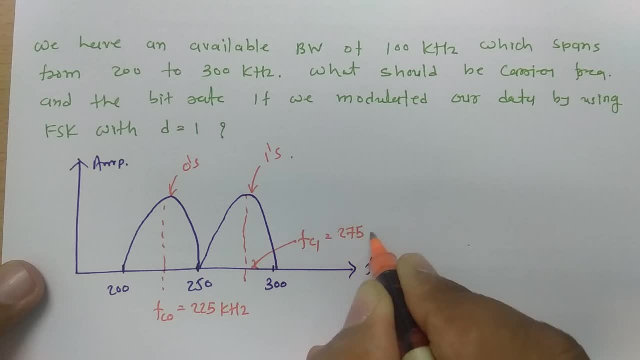 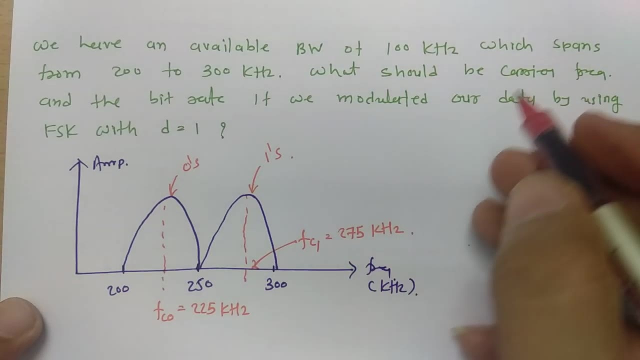 and in between 250 and 300. so that has to be be be 275, 275, 275, kilo, kilo, kilo, hertz, hertz, hertz. now, now, now, we got. what is that carrier frequency? we got, what is that carrier frequency? we got, what is that carrier frequency right? 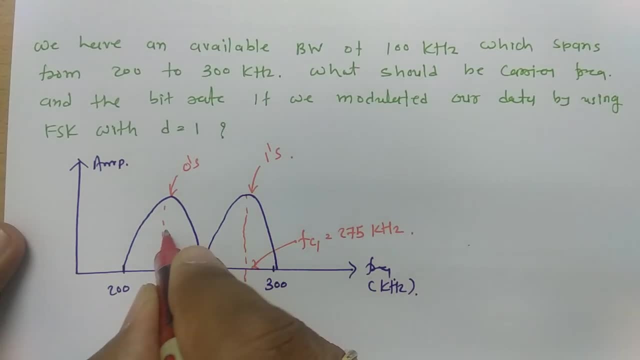 right, right now. one more thing that we need to identify. now, one more thing that we need to identify. now, one more thing that we need to identify, which is, which is, which is two delta. see this gap: that is two delta, two delta, two delta, f, f. now, from this, 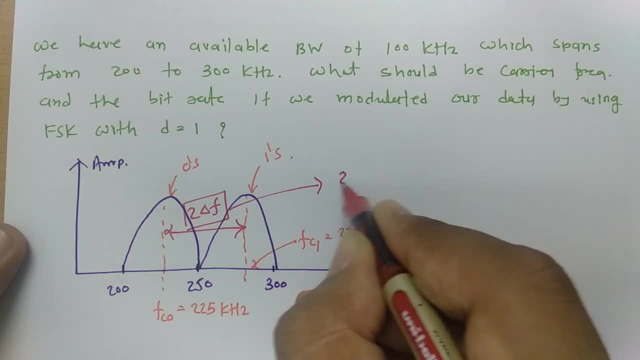 now from this, now, from this gap, we can easily identify gap. we can easily identify gap. we can easily identify 2 delta f that has to be 2 delta f that has to be 2 delta f that has to be 275 minus 225, so that will be. 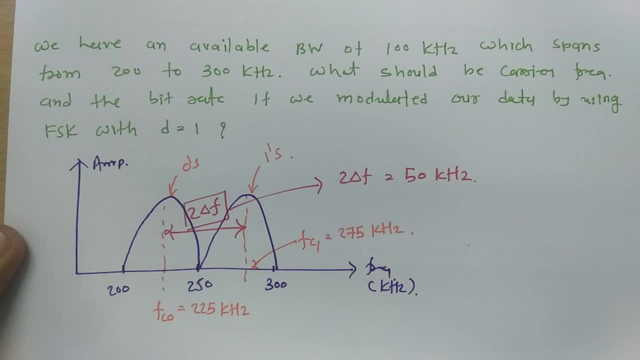 275 minus 225, so that will be 275 minus 225, so that will be 50 kilo, 50 kilo, 50 kilo. hertz, hertz, hertz. so now we have 2 delta f, that is 50. so now we have 2 delta f, that is 50. 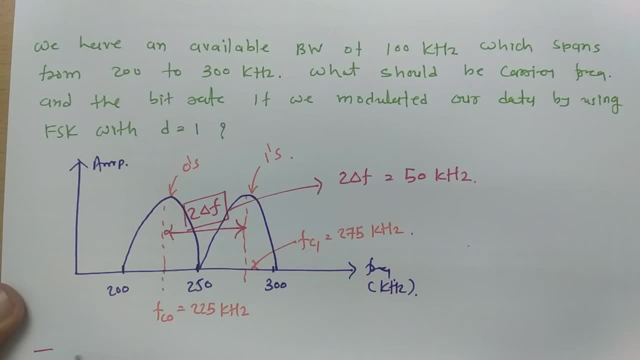 so now we have 2 delta f, that is 50 kilowatts, kilowatts, kilowatts, so so, so bandwidth that is given to us, that is bandwidth that is given to us, that is bandwidth that is given to us, that is 100, 100. 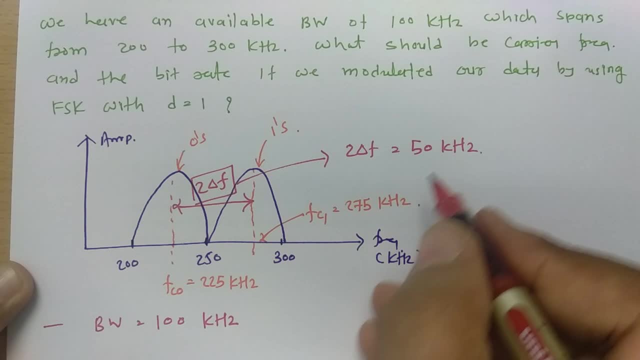 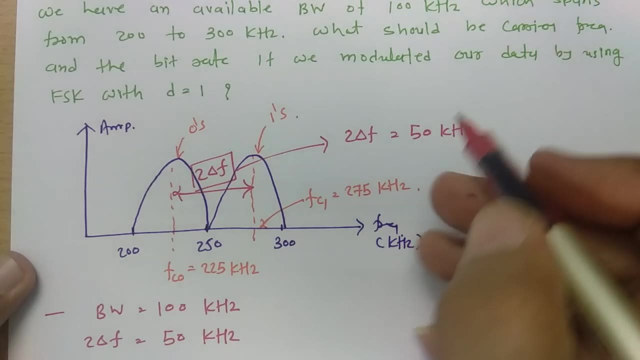 100, 100 kilohertz, kilohertz, kilohertz, 2 delta f that we have identified: 50 kilohertz, 50 kilohertz, 50 kilohertz. so so so question is: what should be the carrier? question is: what should be the carrier? 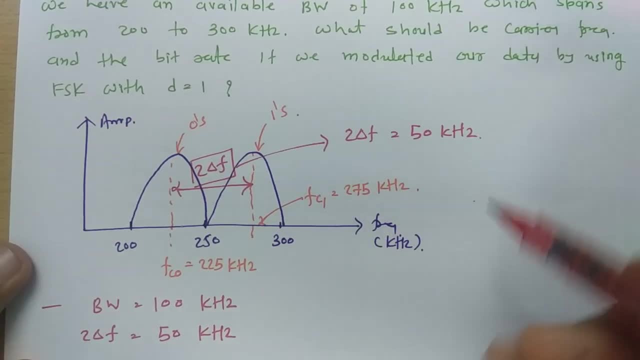 question is what should be the carrier frequency and bit rate frequency and bit rate. frequency and bit rate. so carrier frequency and bit rate that. so carrier frequency and bit rate that. so carrier frequency and bit rate that we are delivered to identify, we are delivered to identify, we are delivered to identify. now see: 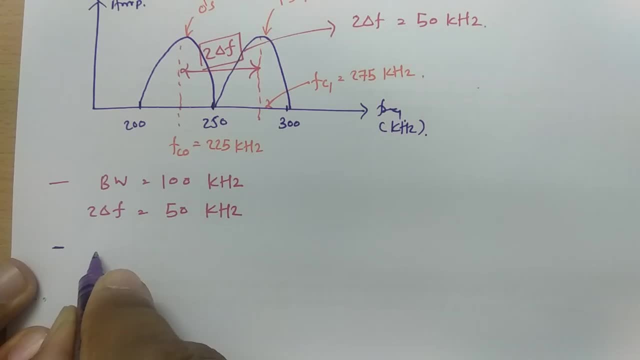 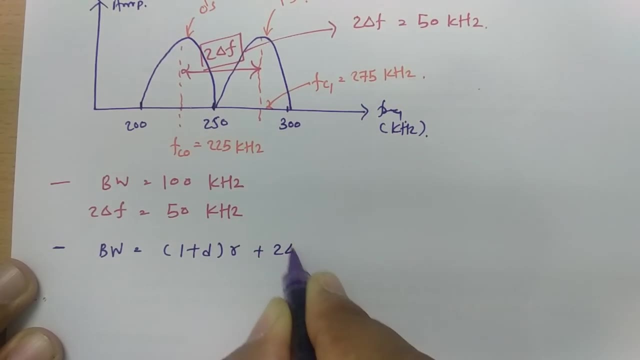 now see. now see for for: for fsk, fsk, fsk, bandwidth, bandwidth, bandwidth that is, that is, that is 1 plus d into r, 1 plus d into r, 1 plus d into r plus 2 delta plus 2, delta plus 2 delta f. 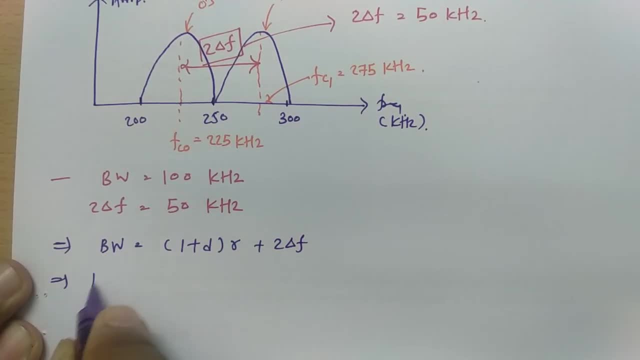 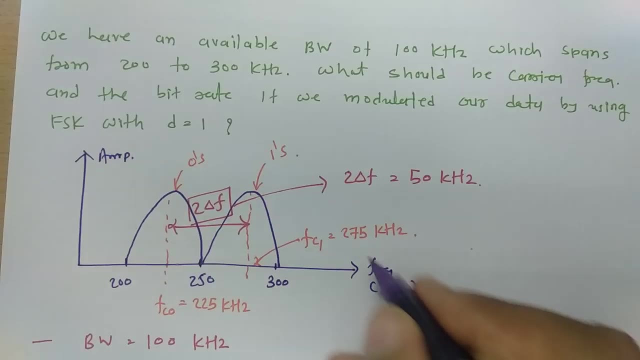 f, f, so here, so here, so here. bandwidth is 100 kilohertz. bandwidth is 100 kilohertz. bandwidth is 100 kilohertz. is equals to 1, is equals to 1, is equals to 1 plus. see in question d is given, that is. 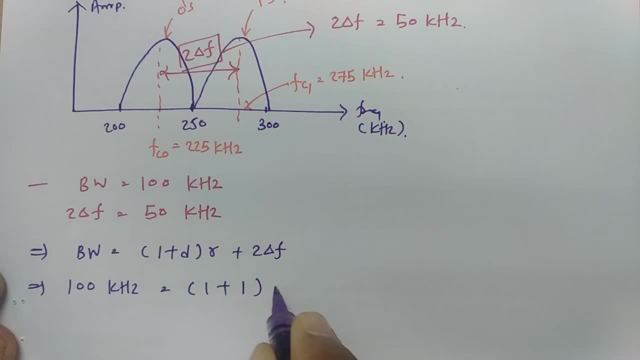 plus. see in question d is given that is plus. see in question d is: given that is 1: 1: 1, so d is 1 plus r, so d is 1 plus r, so d is 1 plus r plus 2 delta f, that is 50. 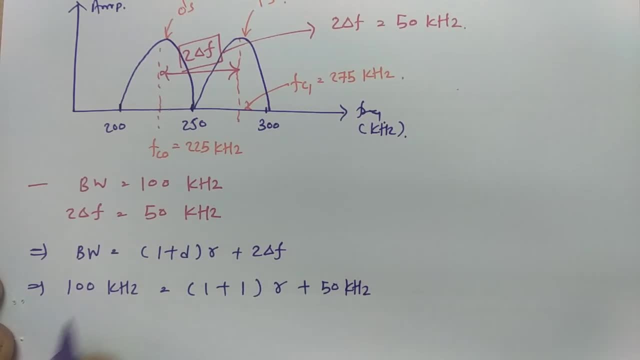 plus 2 delta f, that is 50 plus 2 delta f, that is 50 kilohertz, kilohertz, kilohertz. so if you take this, so if you take this, so if you take this term over this side term, over this side term, over this side, you can say 50 kilohertz. 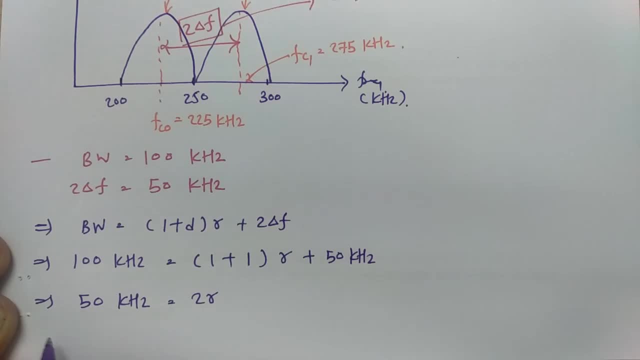 you can say 50 kilohertz. you can say 50 kilohertz, that is equals to 2r, that is equals to 2r, that is equals to 2r, so so so r is equals to 50 divided by 2, that is: 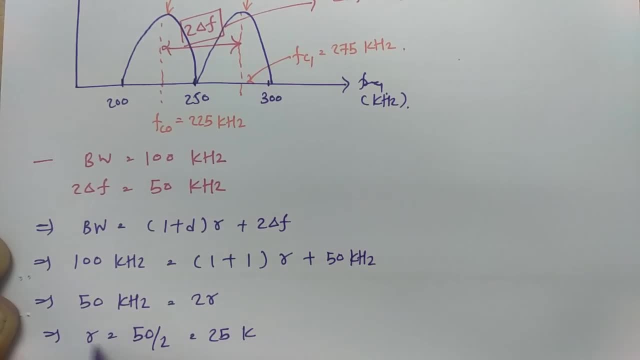 r is equals to 50 divided by 2, that is, r is equals to 50 divided by 2, that is 25, 25, 25 kilo kilo kilo and r is baud rate, so kilo and r is baud rate, so kilo. 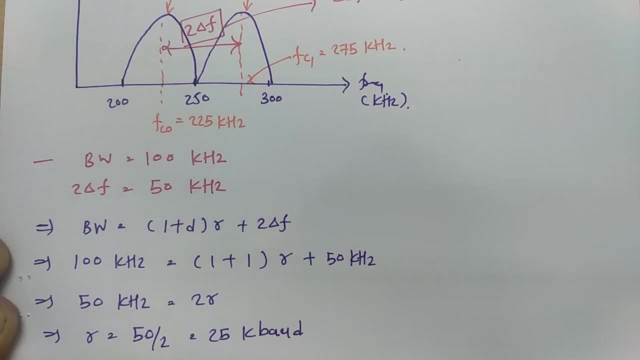 and r is baud rate. so kilo b? a u b a u b a u d baud d baud d baud so r is 25 kilo. so r is 25 kilo. so r is 25 kilo pod pod pod now in the question: 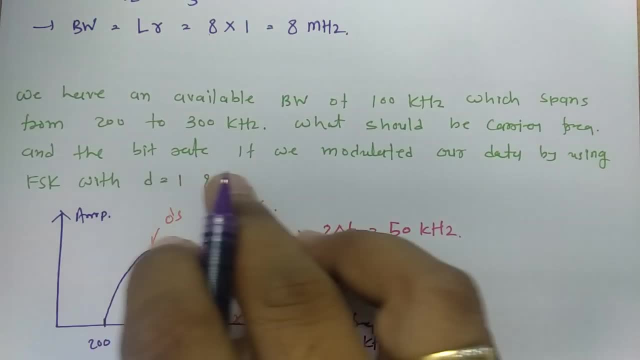 now in the question. now in the question we have, we have: we have been asked with bit rate, been asked with bit rate, been asked with bit rate. so bit rate, that is what we are, so bit rate, that is what we are. so bit rate, that is what we are delivered to calculate. so we have now 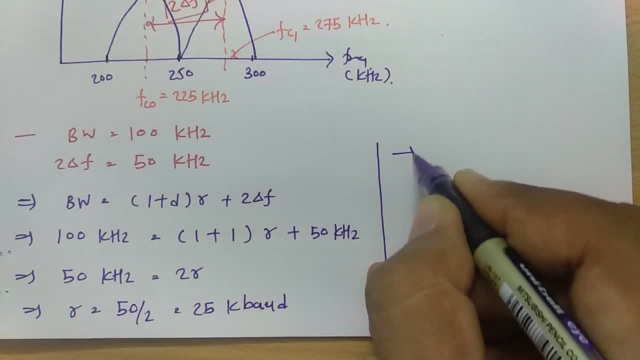 delivered to calculate. so we have now delivered to calculate. so we have now baud rate, baud rate, baud rate. so from baud rate we can have bit rate. so from baud rate we can have bit rate. so from baud rate we can have bit rate. now, what is bit rate and baud rate? 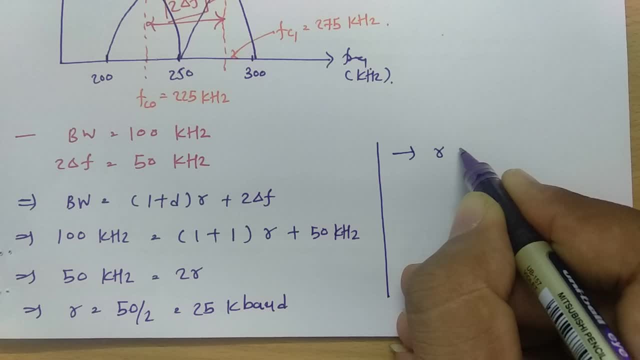 now, what is bit rate and baud rate? now, what is bit rate and baud rate relation, relation, relation, so bit rate and baud rate. that is so. bit rate and baud rate, that is so bit rate and baud rate that is related by. r is equals to capital r by. 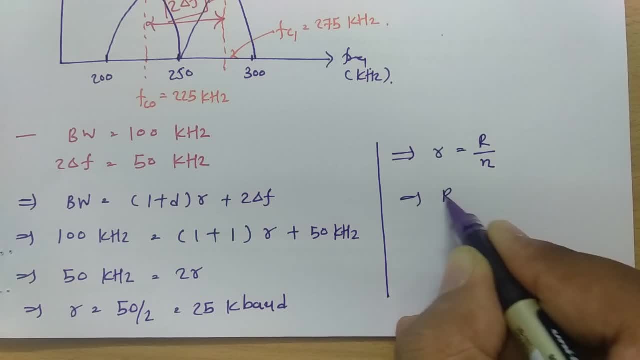 related by r is equals to capital r by related by r is equals to capital r by small n. so from that we can have capital small n. so from that we can have capital small n. so from that we can have capital. r, that is n into, r, that is n into. 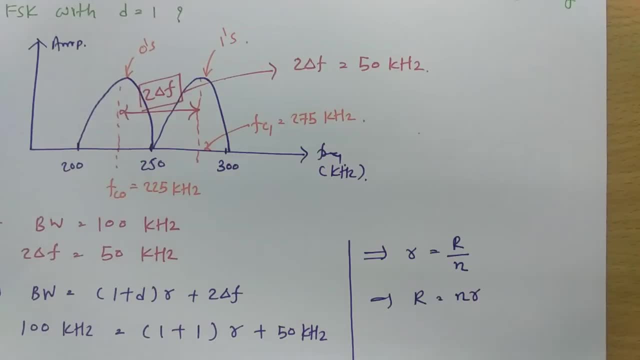 r, that is n, into smaller. now see smaller. now see smaller. now see here: two level fsk is given. here two level fsk is given. here two level fsk is given here. two level: here two level fsk is given. here two level fsk is given. 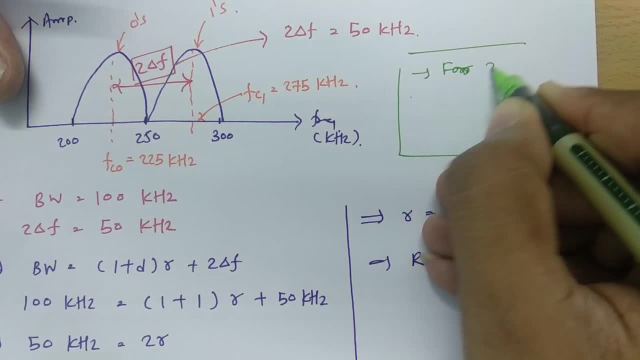 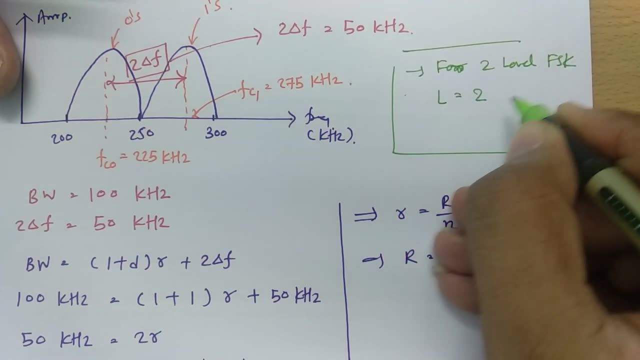 here two level fsk is given, given, given, given, so for so for so, for two level, two level, two level fsk, we can say fsk. we can say fsk. we can say l is equals to two, l is equals to two, l is equals to two if you compare this with two to the 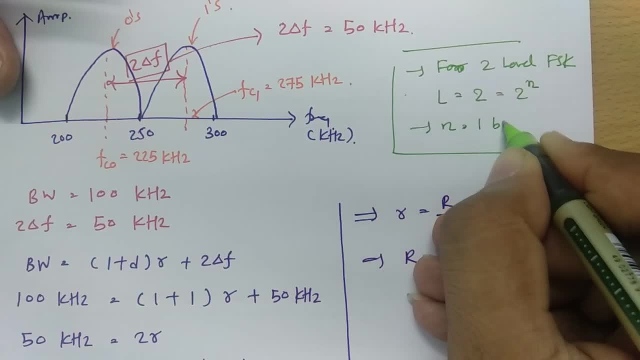 if you compare this with two to the, if you compare this with two to the power n, then you can have: n is equals to power n, then you can have: n is equals to power n, then you can have: n is equals to one bit, one bit, one bit. so for two level fsk, n is equals to one. 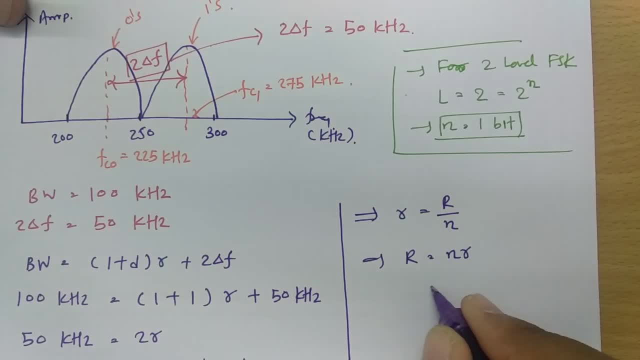 so for two level fsk n is equals to one. so for two level fsk n is equals to one, bit, bit, bit. so if you place values, so if you place values, so if you place values, n is equals to one, n is equals to one, n is equals to one, and 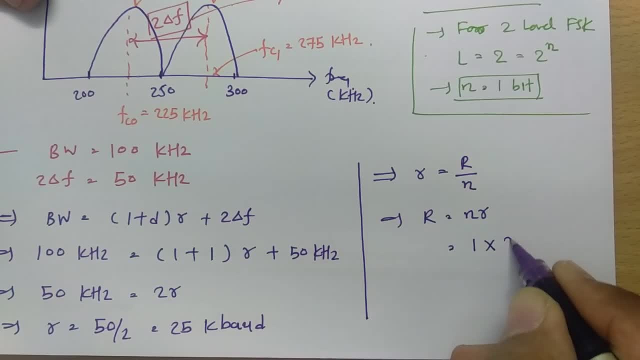 and and. r is equals to 25 kilobaud, r is equals to 25 kilobaud, r is equals to 25 kilobaud, so 25, so 25 so 25. so that will be 25 kilobits, so that will be 25 kilobits. 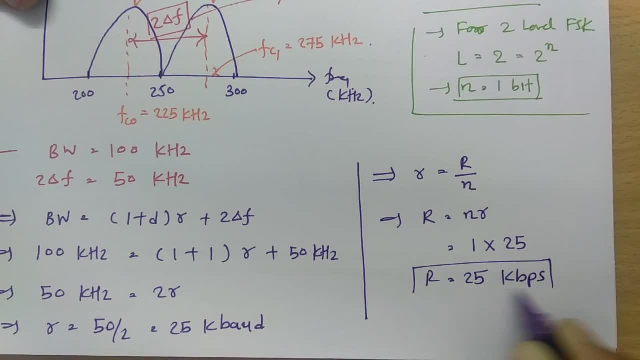 so that will be 25 kilobits per per per second. so data rate that will be kilobits second. so data rate that will be kilobits second. so data rate that will be kilobits per per second. so whenever you are been asked with this, 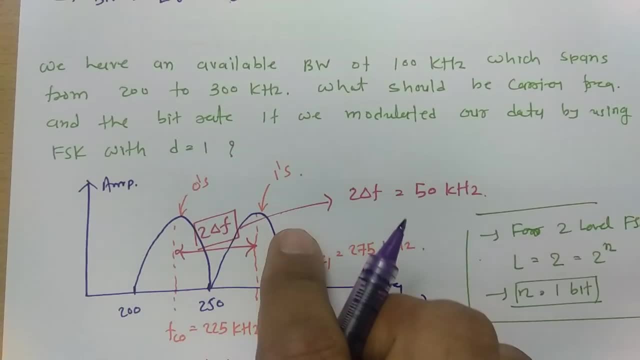 per second. so whenever you are been asked with this per second, so whenever you are been asked with this kind of problem, kind of problem, kind of problem, you just draw a spectrum first. that will you just draw a spectrum first. that will you just draw a spectrum first. that will gives you idea about what is that. 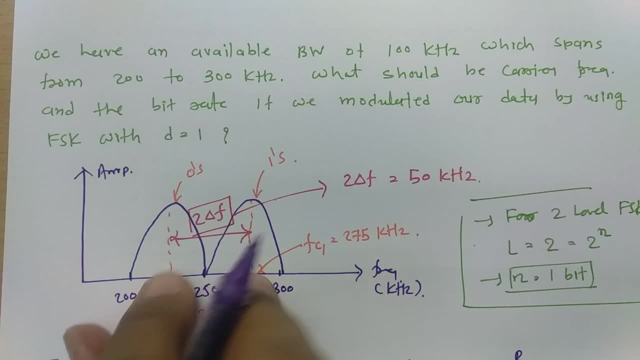 gives you idea about what is that gives you idea about what is that delta two delta f. gap in between two delta. two delta f gap in between two delta two delta f gap in between two bands, bands, bands, and once you have two delta f band gap and once you have two delta f band gap. 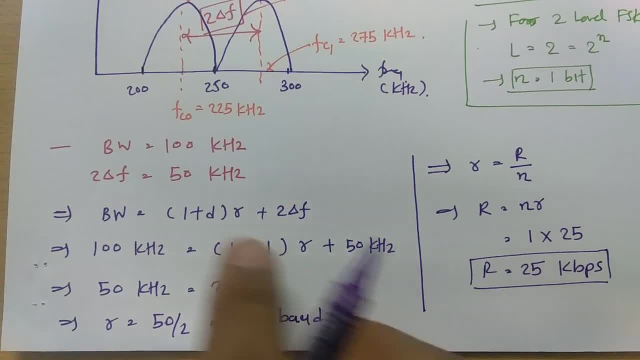 and once you have two delta f band gap in between two bands, in between two bands, in between two bands, you can apply that to basic formula of, you can apply that to basic formula of, you can apply that to basic formula of bandwidth and that basic formula of.